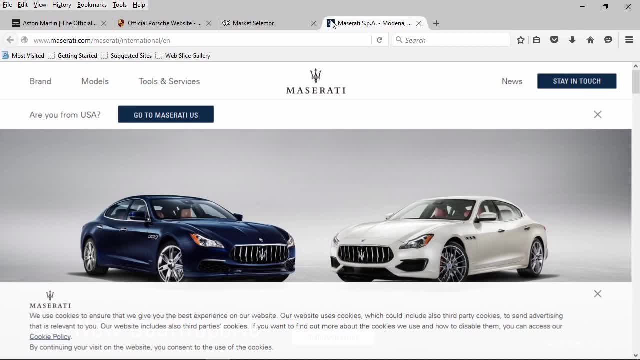 gone to my browser and I'll go to my theme of cars. So I'll go to my theme of cars, So I'll go to my multiple websites. So now what we want to do is we're going to look at these websites Remember. 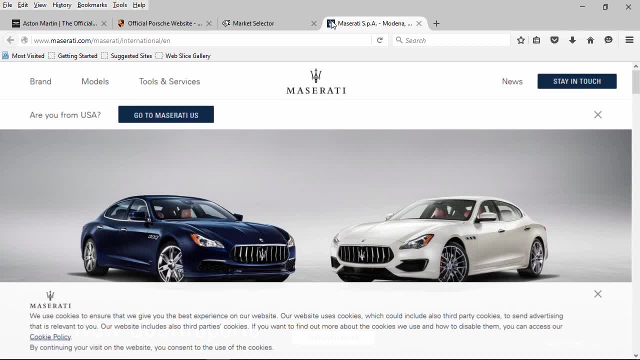 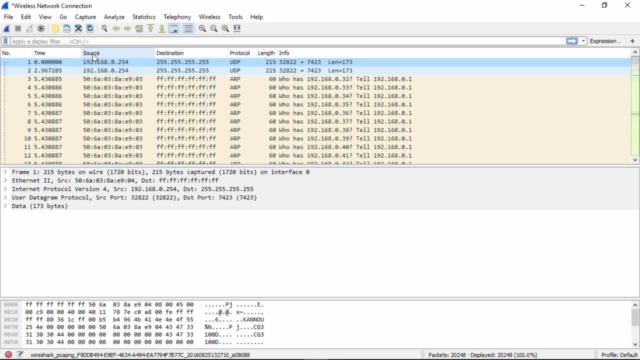 if you're following along, you can use any websites you want and the process is going to work. And that's the key- is the process. So now I'm going to actually stop my packet capture. So what we're going to do is: I want to go all the way up to the top here at packet one, and we got our UDP. 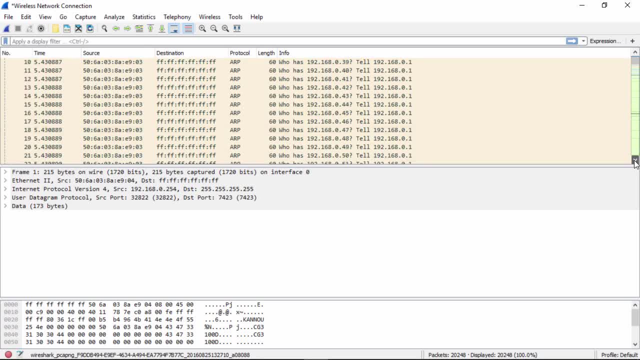 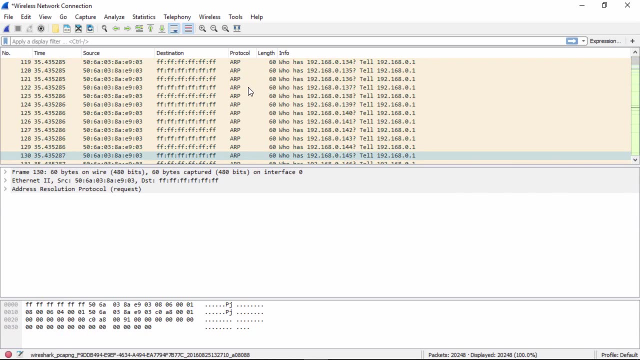 which is our SSDP, and we got all this ARP traffic which normally you wouldn't see on a network. So I have to investigate that. Something's going on with my cable router so I'm not going to worry about that right now And as I go down here I'm looking for the UDP traffic. So we know. 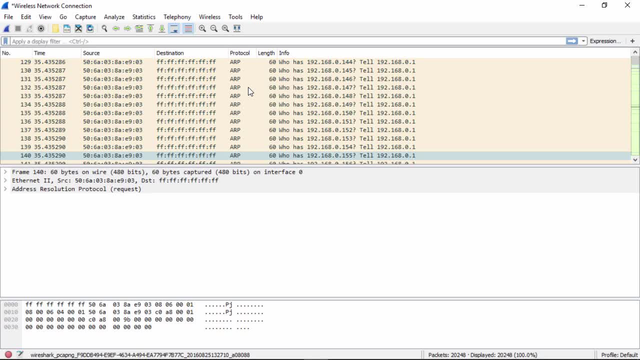 we want is a DNS query for our network traffic. There's a number of other DNS queries. So the first steps we want to review the communication parameters. We look for the DNS and then move to the packets. There are different ways to do this. I like to use the bottom. 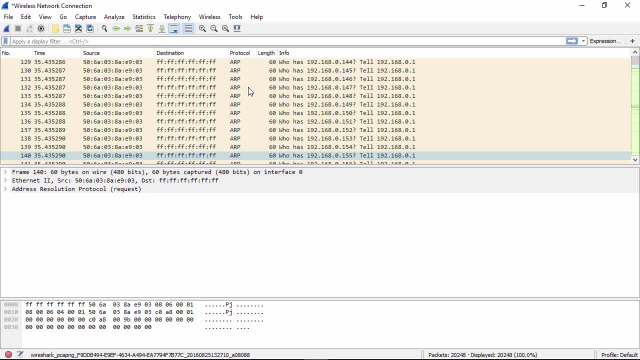 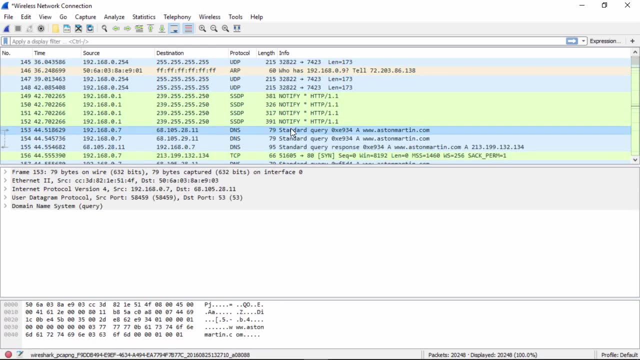 bottom window and it comes with practice. But as you look at practice and you do things, you get used to exploring the network traffic. So again, there's my Aston Martin, So there's my query for astonmartincom. So remember, after I get the DNS query, shouldn't take that long to. 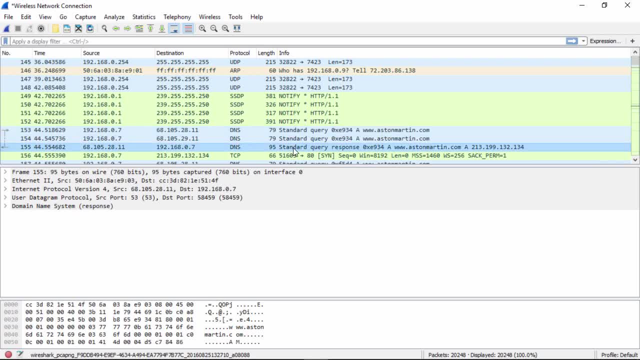 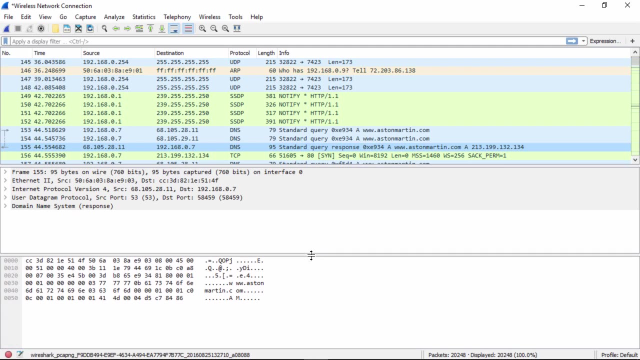 get the response. There's the response. Immediately following this I get information for the connection. So it comes with practice. but more we look to work at it, you'll get better at it. So I said there's different ways of doing this. I'll pull this bottom window up So we have it here in the 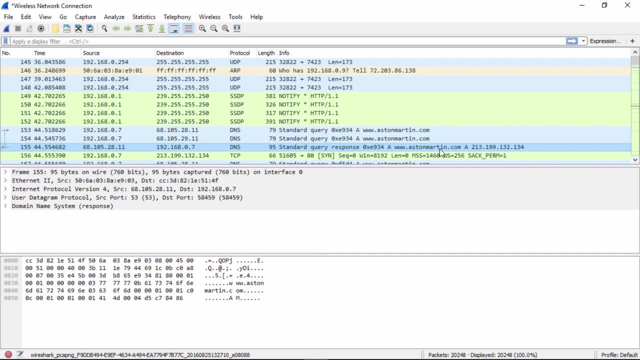 information block of the upper window or the top window for the Wireshark tool, But we're also have it down here in the details block, which is the hexadecimal dump. So we got it either place. So which one you use is entirely up to you, of course. But now we have the IP address of Aston Martin. 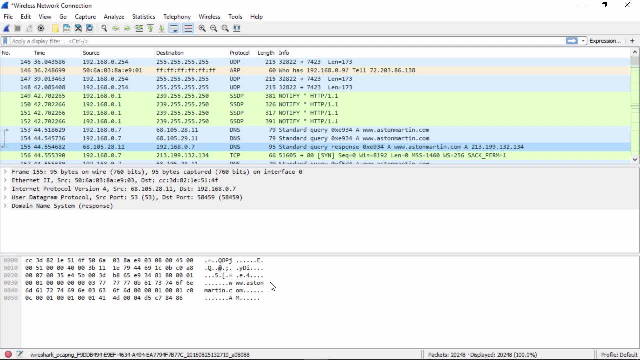 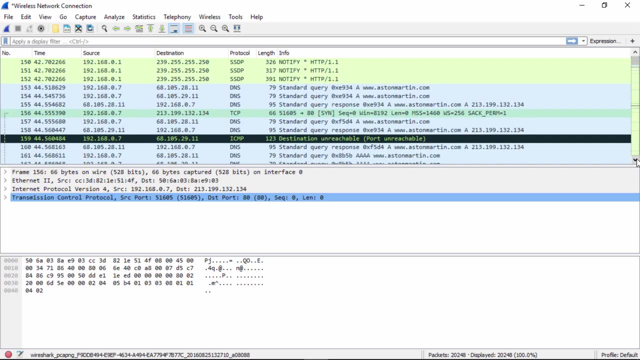 All right. So we have a lot of different things. So this is the Aston Martin, So it's not encrypted. If it was encrypted, I wouldn't be able to read it, But in this case we see the send packet- in this case for Aston Martin, in the three-way handshake- is going to port 80. So HTTP. 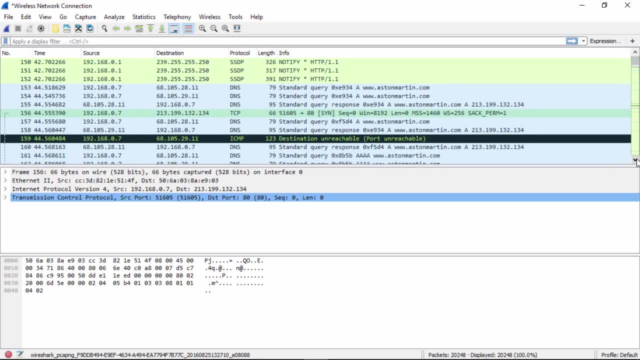 hypertext transfer protocol. So all I'm doing is looking for anything that might be of interest. Remember, in the static capture file we had FTP traffic across that. with FTP file transfer protocol the data is in clear text. so here what we're looking for is the data with Aston Martin. so now I just right. 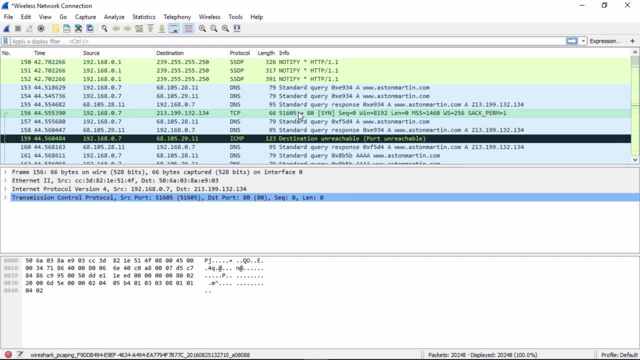 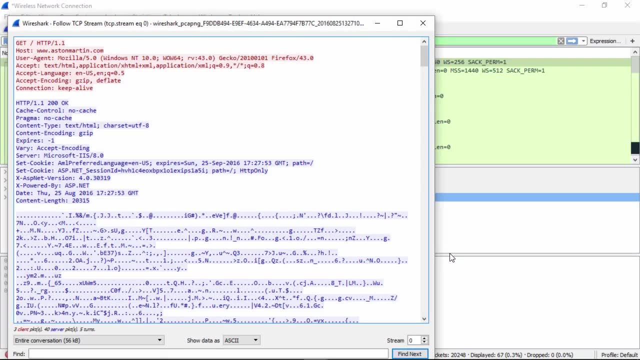 click the send packet which is right here after the query, and I use my methodology of following the stream. so now we get in here and we have information. remember, red is the client, blue is the server, and we see right in here, we see what, we see that they're running on their server. Microsoft IIS 8.0. 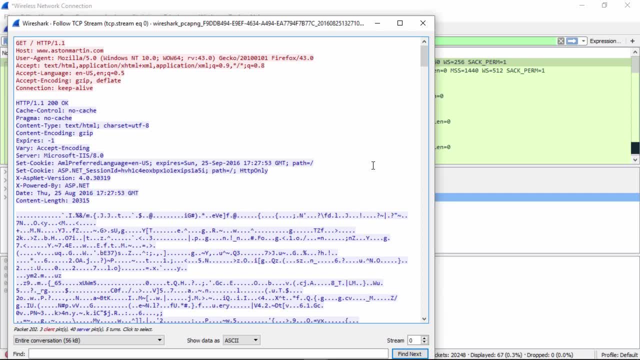 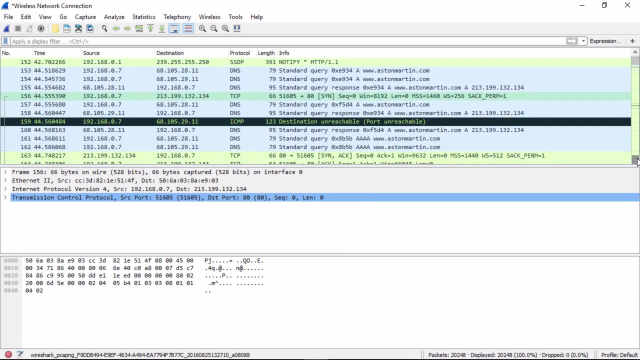 so again, this is all data and information we've been able to obtain because we have a process and methodology for doing protocol analysis. so now, if I close out of this, I clear my filter and I continue my little quest. so I scroll down again. that's my Aston Martin. 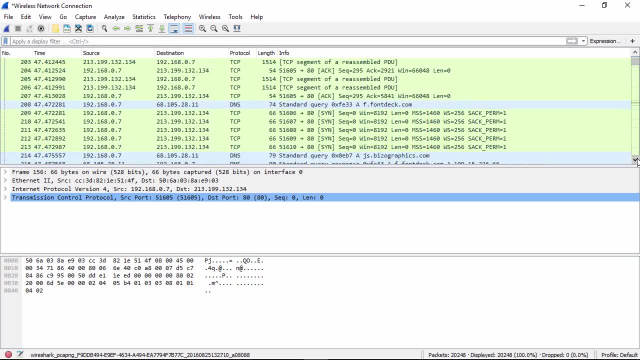 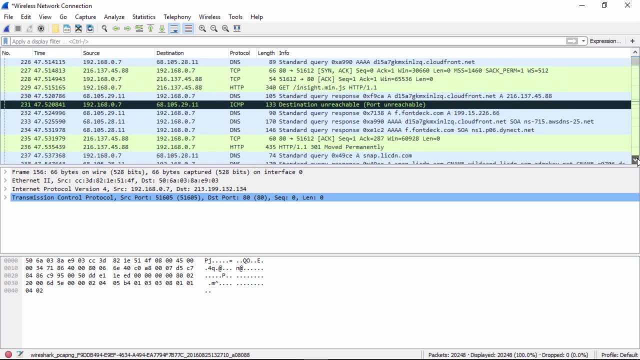 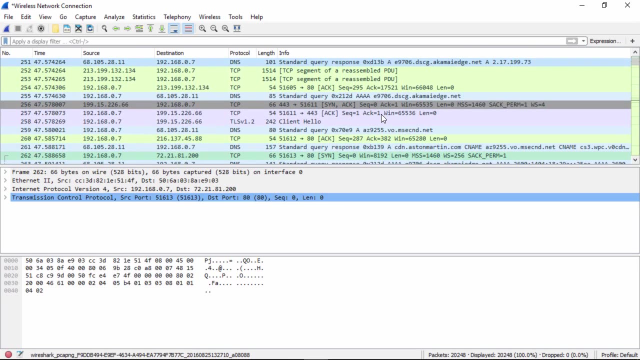 and I will show you quicker ways to do this, as we go through in different things, and there's all this stuff that comes along with going to a website. as I said, unfortunately that's all part of your data mining, so we keep coming down here and we'll learn. filtering is the way to do this quickly and we'll learn. 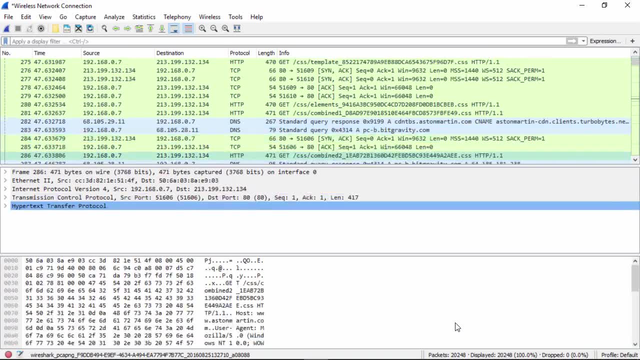 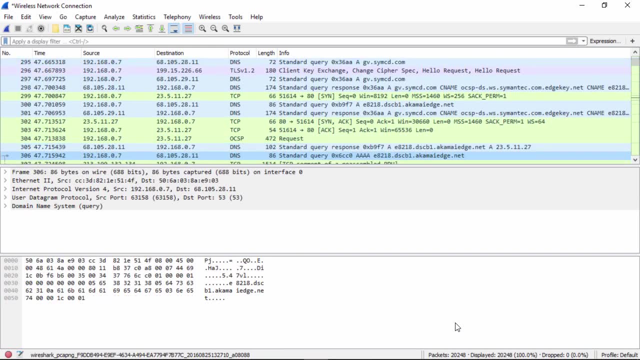 that once we get into more analysis. and again, as I said, all this information is what's taking place every time you connect to the internet. it's why, if you've ever went and you've done a shopping and you've bought something or just looks for something online, 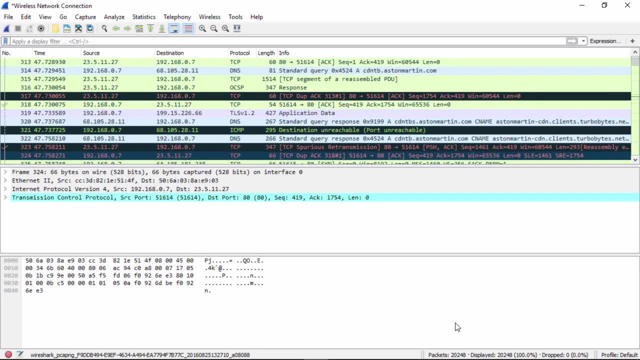 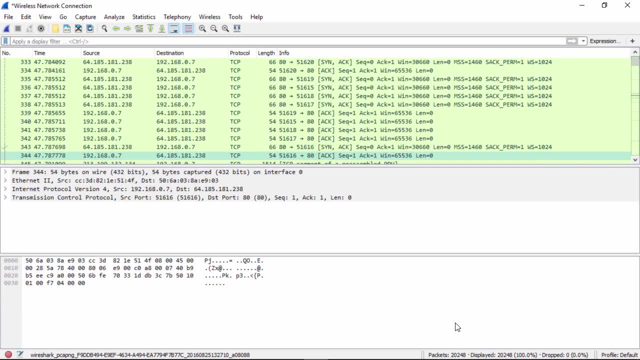 curiously, every time you go online you'll start seeing those types of things. the best example of that: I had an actual. I needed a computer laptop bag. mine broke when I was on travel one time, so I was looking one night trying to find one in the next three days all I seen was a. 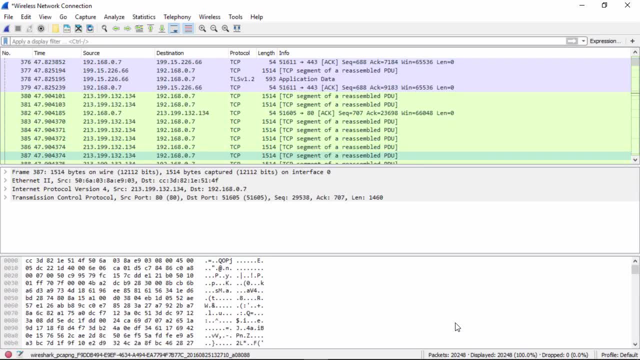 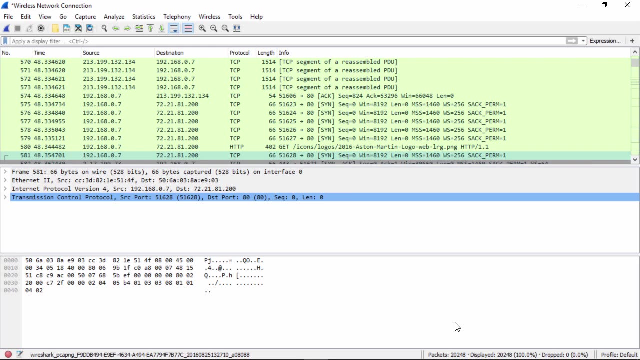 advertisements for luggage, laptop bags and luggage. so again, it's all data mining. data mining has taken place every time we go on the network today. this is what we're looking here in the network traffic. you're looking at all the things taking place at the network level. this is why it's so important to 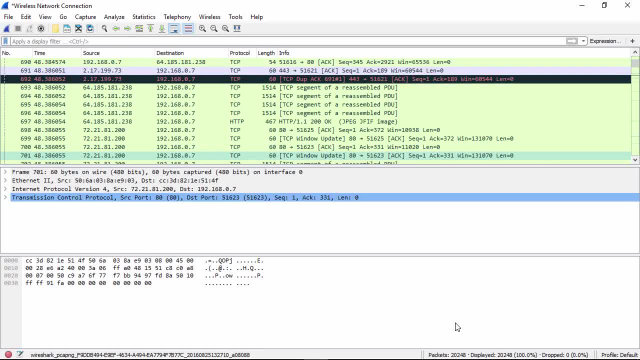 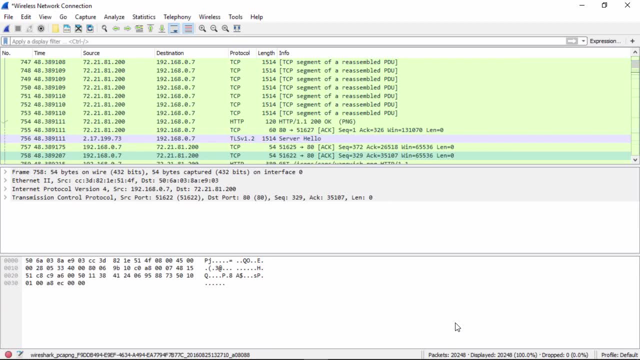 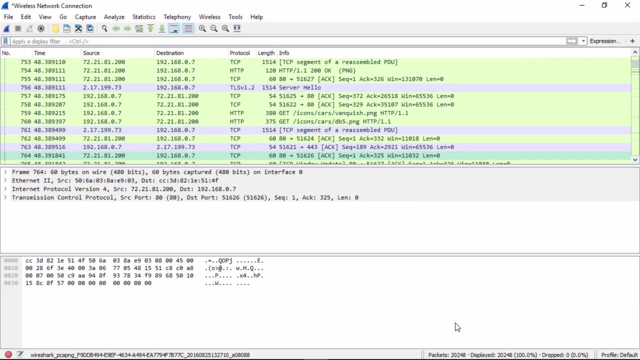 understand how to do protocol analysis. alright, so different types of things. so once you've had the process, now you can look at different things. and again, as I said, we're looking at different things. and again, as I said, all this information is We will start looking at this traffic with a process and methodology that allow us to give us filter. 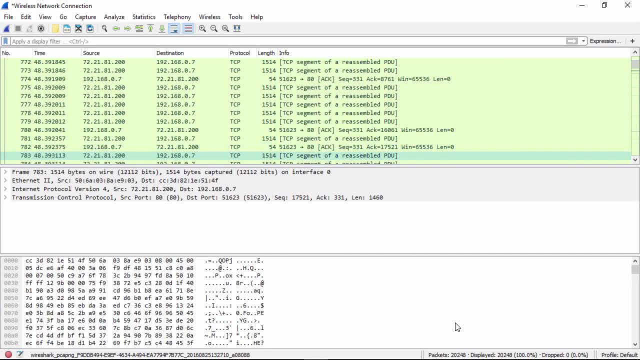 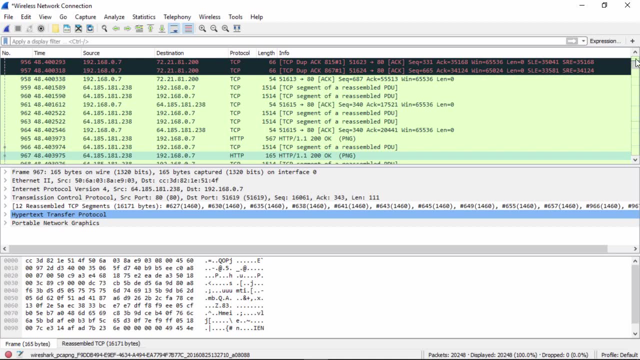 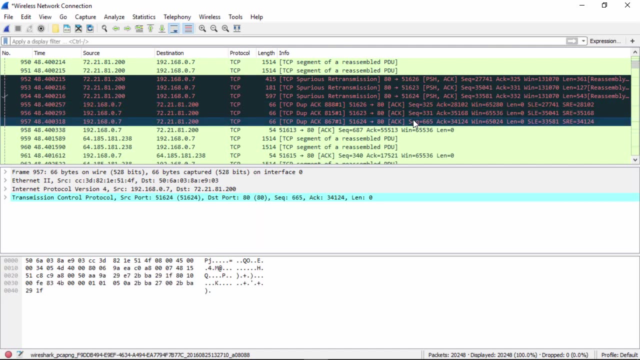 A lot of different filtering information. All right, So a lot of things on this network. So as I scroll down, I'm just looking for any suspicious. Now I got some suspicious traffic coming up here, So now the Wireshark tool is helping me telling me: hey, you got some duplicate, duplicate acknowledgements. 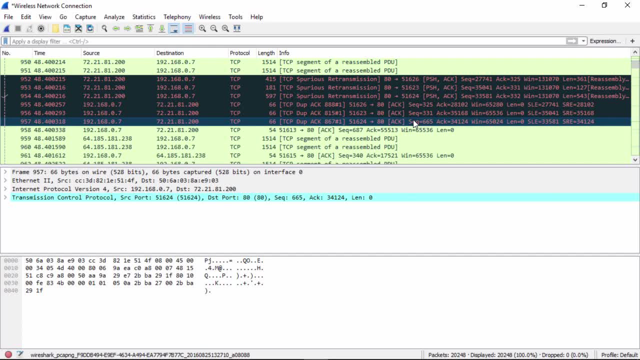 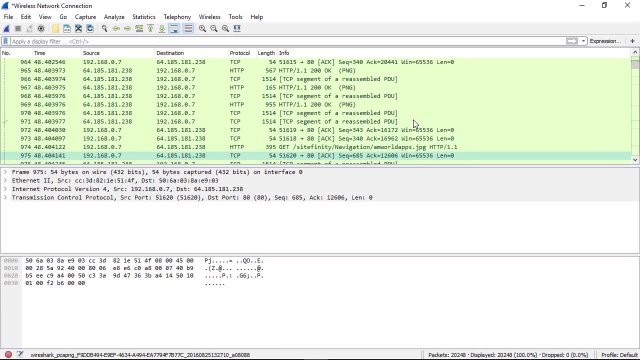 Well, that could be a spurious retransmission, as it says here. Again, it would require more investigation, But in most cases it's probably just noise on the network, because we have a lot of noise on any of our networks today. 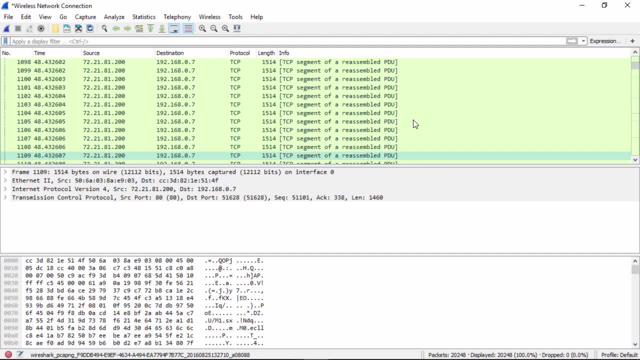 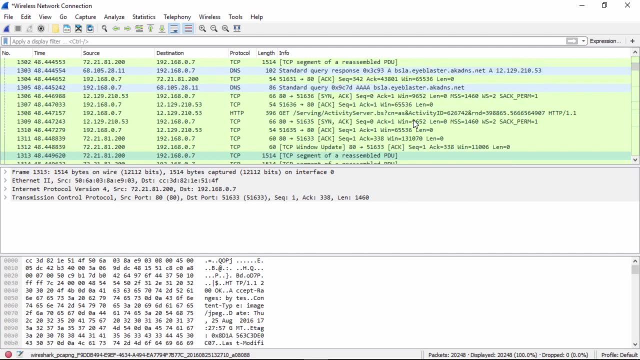 Because, again, data mining. all this comes from data mining. So, as you see here, all this noise is taking place on the network. Now, once we get into the next section, we'll teach you how to filter this and only look at specific components. 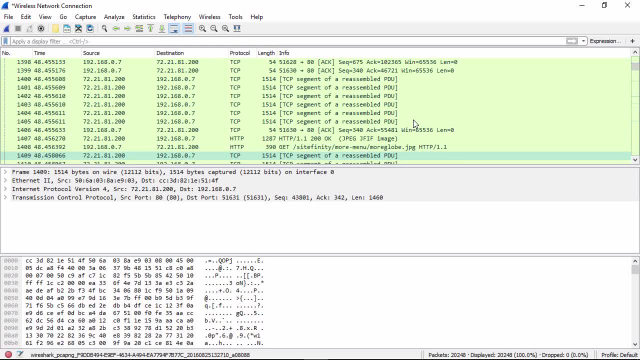 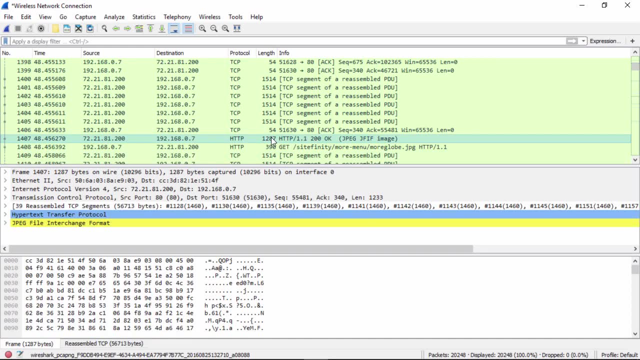 of what's taking place on the network, And that's one of the powerful things to do. So if I go here and just click on an example in this HTTP which is a JPEG, So in this case there's a JPEG file coming across. 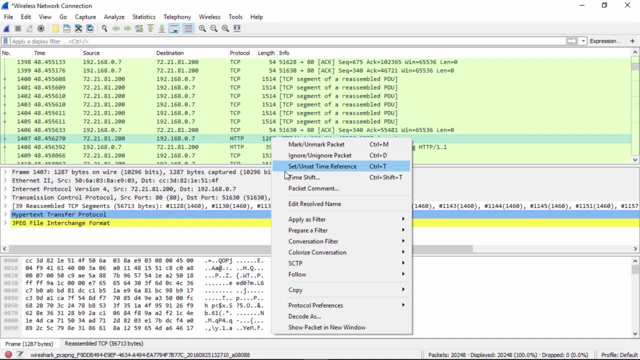 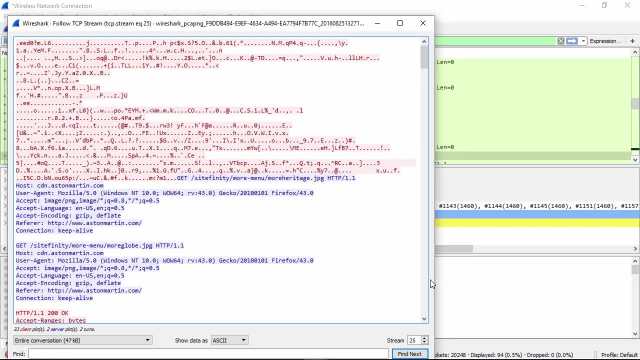 So now, if I apply my methodology, identify the TCP traffic or UDP traffic, right-click it, select Follow TCP Stream. Now there's all the data there, And this again is Aston Martin, CDN, Aston Martin. So this is a little bit of a trick. 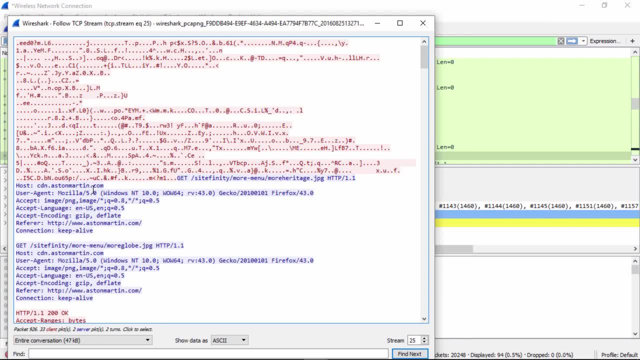 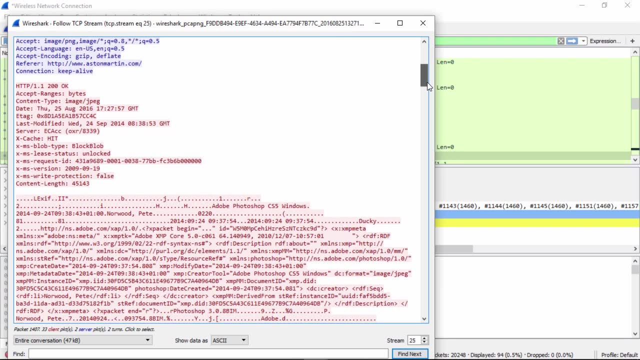 So this is a little bit of a trick. This is a little bit different Aston Martin than the Aston Martin I looked at before And it's a referrer from Aston Martin. So if we scroll through here we have all kinds of information that's taking place. 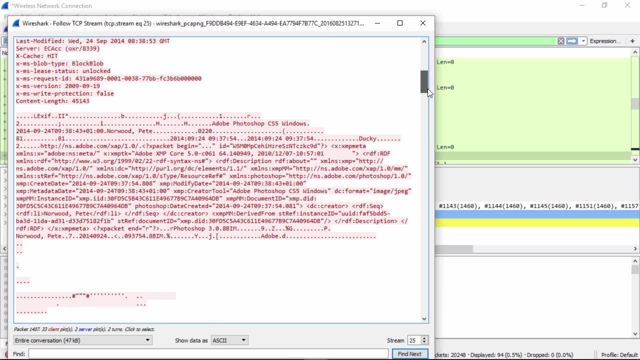 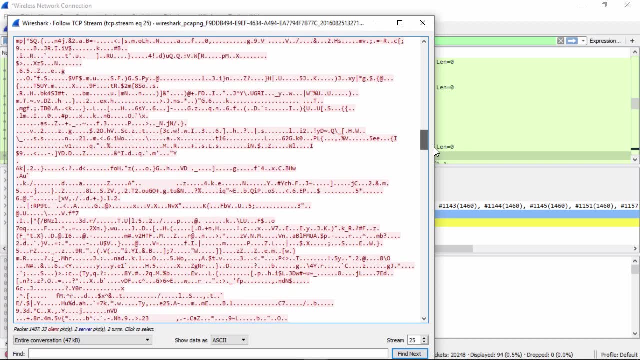 We even got this Adobe Photoshop and we got this guy, Norwood, Pete Norwood. We got all kinds of stuff in here: Adobe, all kinds of data. Again, this is nothing but network traffic that's taking place between my machine and, in this case, 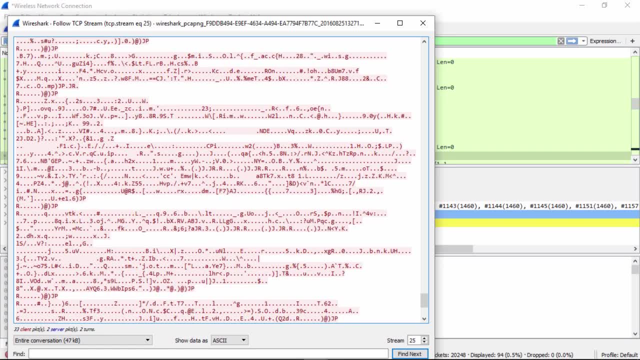 the Aston Martin server. So that's the power of doing this stuff. You actually learn how to actually do protocol analysis. What protocol analysis does is teaches you what's taking place on the network. So as you build your skills, you'll get more familiar with this. 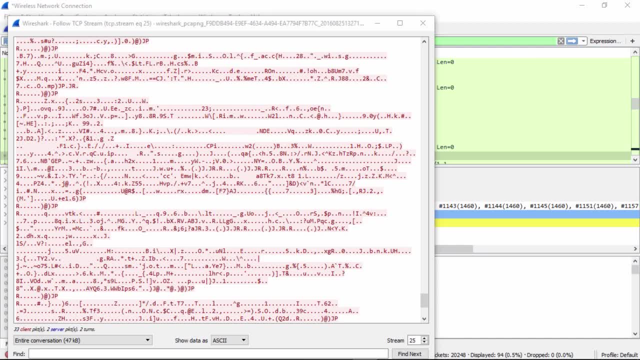 And, like anything else, you got to practice it over and over again until you get proficient at it. That's how we learn. Next up, we'll continue. We'll work with capture files. We'll work with the Aston Martin server. You'll get a variety of different functions closely aligned. 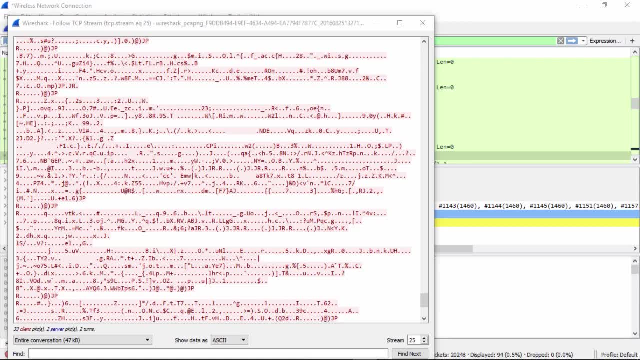 You can monitor the networks and �ار샵 tools themselves within the Wireshark tool And explore more ways you can filter that data to make it more granular so you can get a good look at what's taking place on the network. 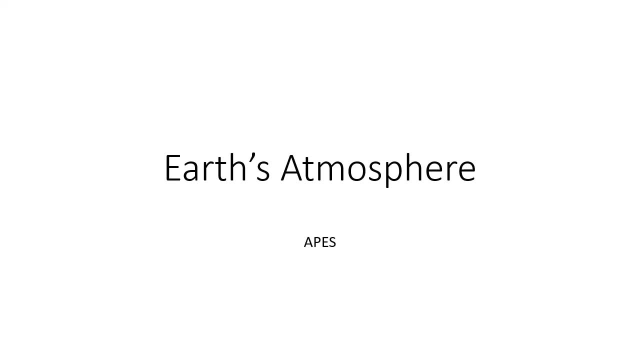 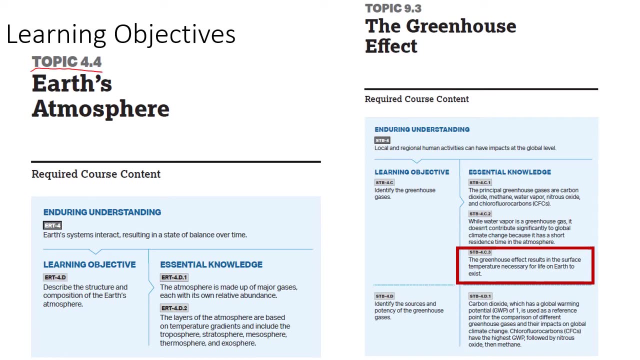 Welcome everyone. This PowerPoint is AP: Environmental Science- Earth's Atmosphere- The learning objectives. we're going to focus on topic 4.4, which is Earth's Atmosphere- The enduring understanding. Earth's systems interact, resulting in a state of balance over time. 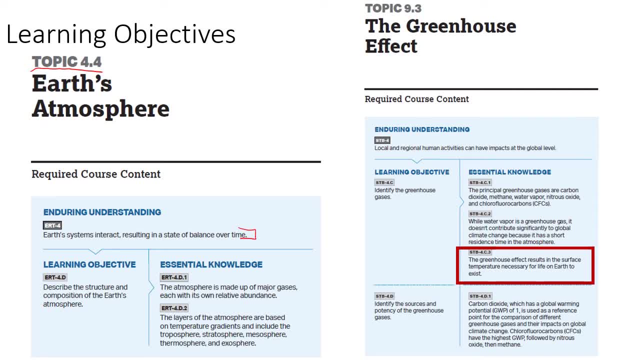 This is the same enduring understanding as the last one, where we talked about tectonic plates. The learning objectives describe the structure and composition of the Earth's atmosphere. This is what we're going to stay with most of the time, and we'll talk about the essential knowledge. 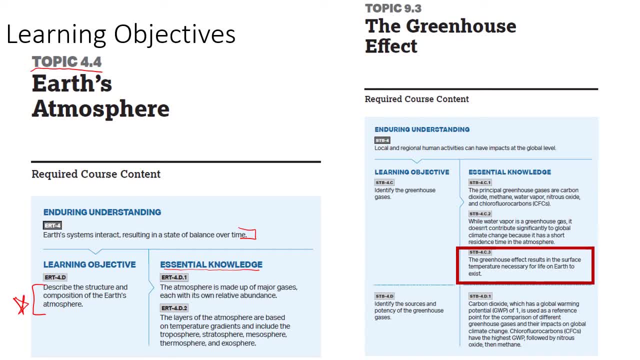 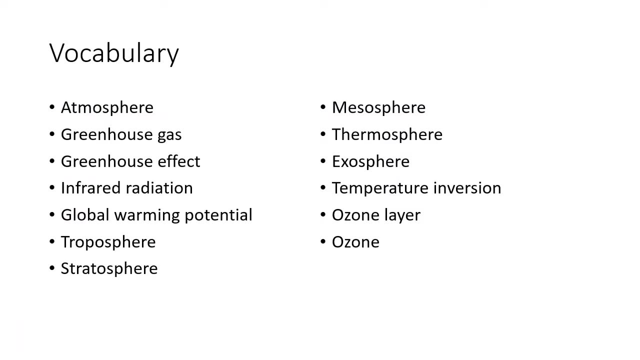 um, at the end, as usual, We're also going to touch on one other learning objective. This is topic 9.3, the greenhouse effect, and we're really just going to talk about this one: what the greenhouse effect is and what it results in Vocab. as usual, I'm going to skip, but you can. you can pause this.